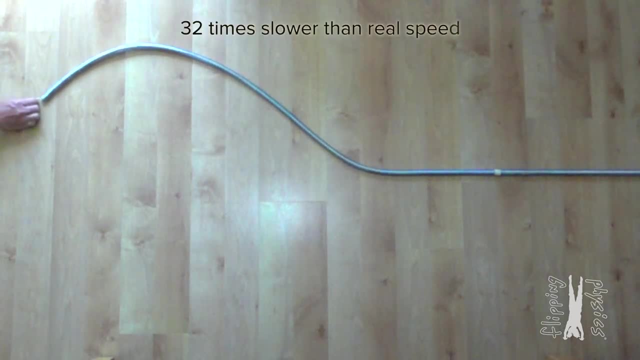 Which is why I have slowed it down: 32 times slower than real speed. Again, this is a single wave pulse moving through a medium. Bobby, what is the medium through which the wave pulse is moving? The wave pulse is in the spring, so the medium the wave pulse travels through must be the 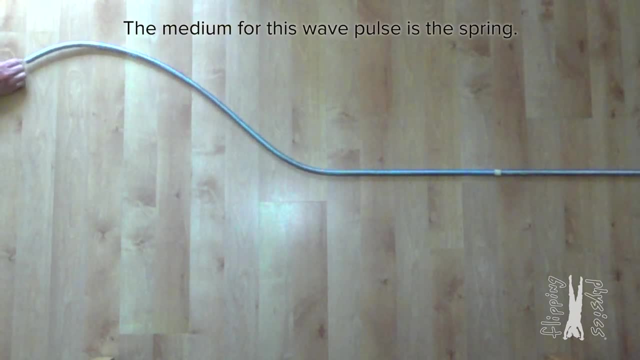 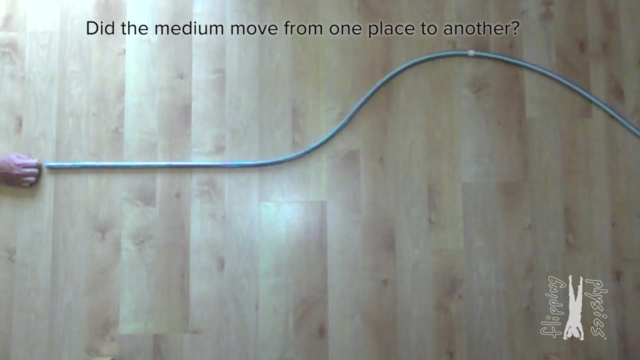 spring. right, Bobby, that is correct. The medium for this wave pulse is the spring. Remind me, class after the wave pulse goes by. did the medium move from one place to another? No, Then class what actually moves through the medium. 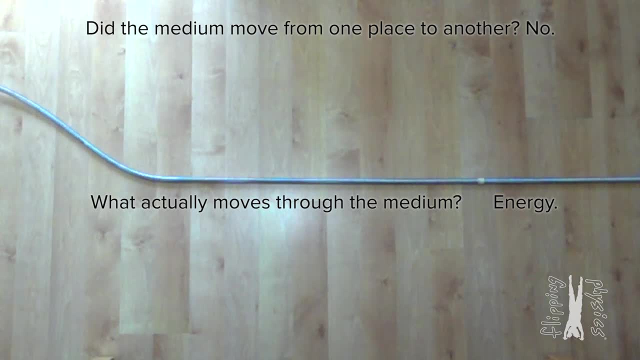 Energy, But it looks like the spring moves, so that does not make sense to me. Okay, Bobby, let's follow the motion of the piece of tape, which is on the spring and therefore is a part of the medium, As the wave pulse travels along. 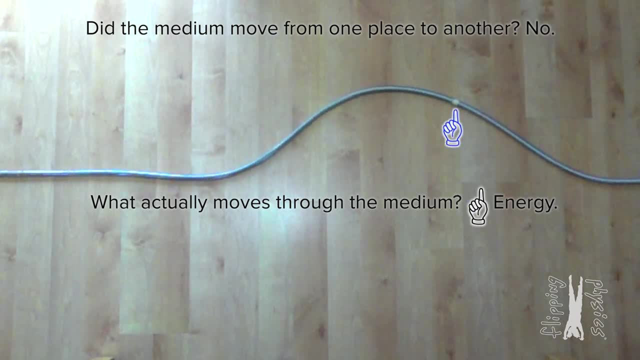 the spring the tape does move. However, the overall displacement of the piece of tape is pretty darn close to zero because the medium does not change locations. Bobby, does that help? Yeah, I can see. the overall displacement of the spring is almost zero. Thanks, 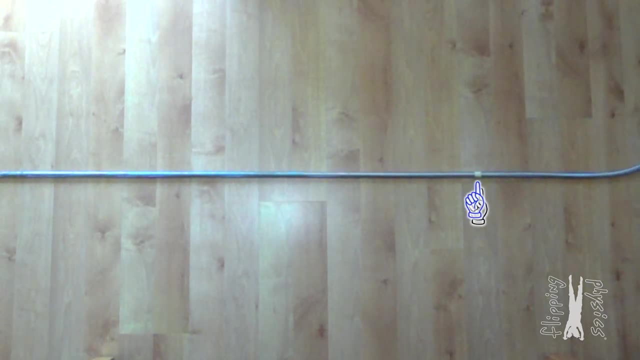 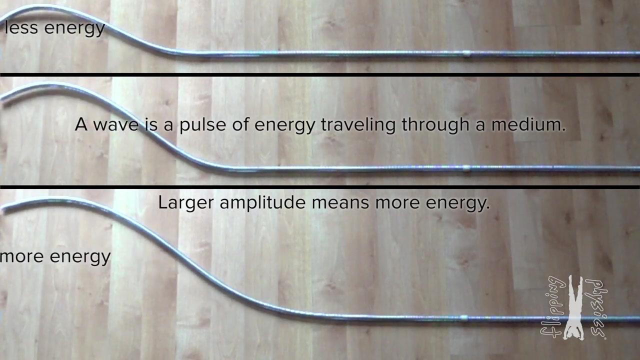 Right. The energy contained in the disturbance of the medium travels along the spring. In other words, the wave is a pulse of energy traveling through the medium. That makes sense. And I bet the larger the amplitude of the wave, the more energy contained in the wave. We know amplitude is the maximum. 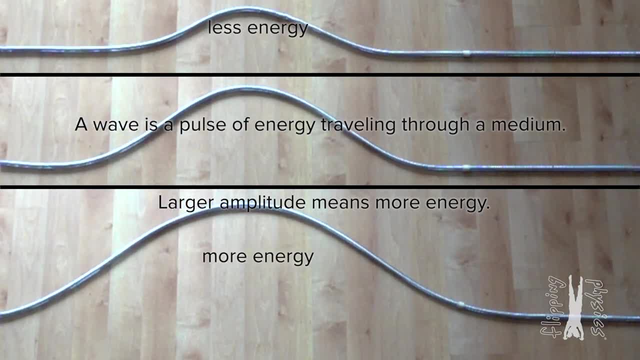 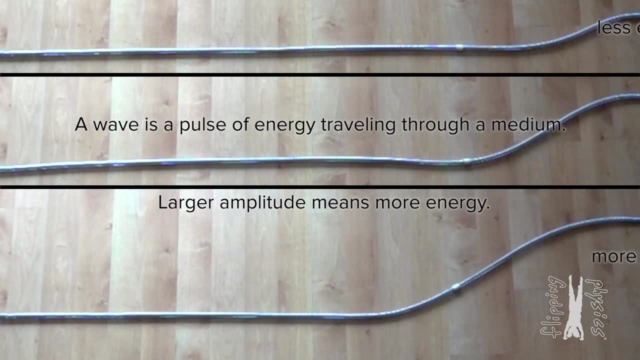 displacement of the wave from equilibrium position. Does that mean we can treat the equilibrium position as the position of the medium, Or is it sort of a badP sir? Good question. the position of the medium before and after the wave passes by a point or where the spring. 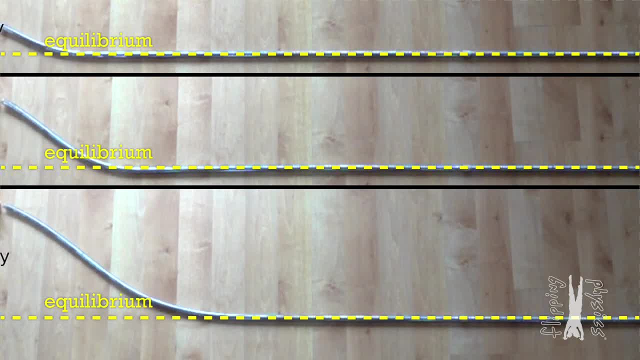 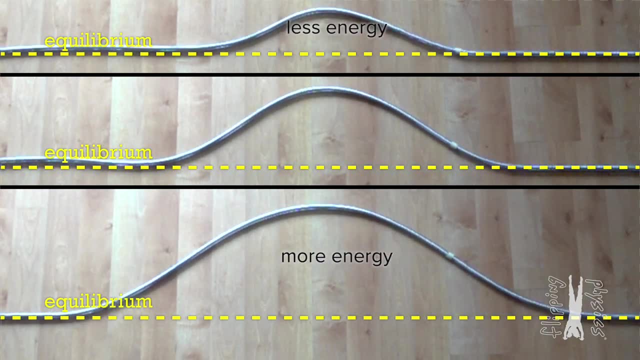 is before and after the wave is there, Mrp, Y'all are correct. A larger amplitude means more energy, and where the spring starts and ends is the equilibrium position, And I bet a larger amplitude wave has more energy because your hand has to do more work. 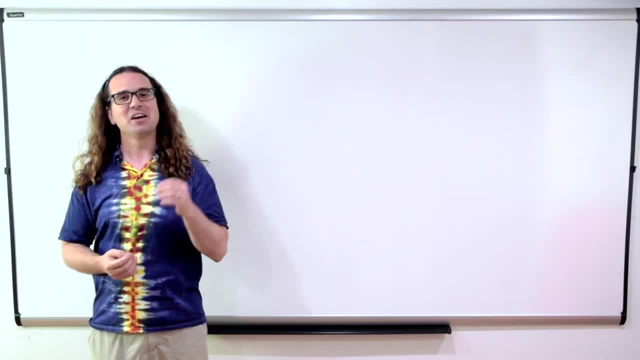 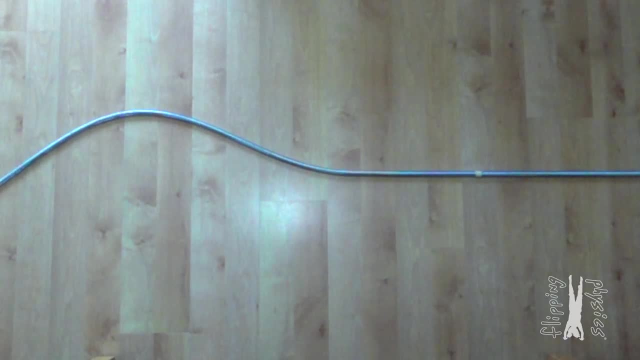 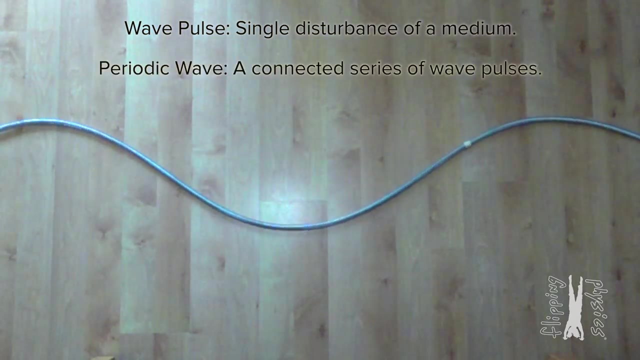 to give it that amplitude right, Mrp? Yes, very nice, Bobby. Okay, what we have shown so far is a single wave pulse. We can also have something called a periodic wave. A wave pulse is a single disturbance of a medium, whereas a periodic wave is a connected series of wave pulses. A periodic 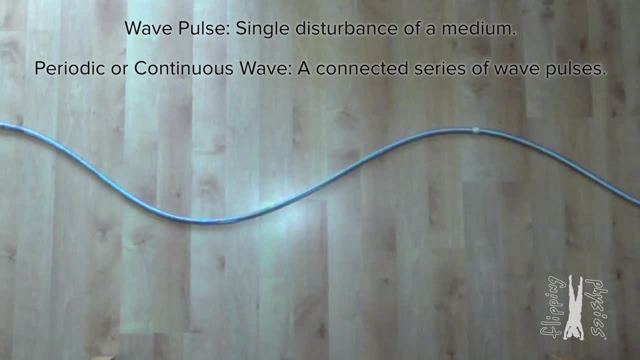 wave is also sometimes called a continuous wave. Okay, a wave pulse is a single wave, and a bunch of wave pulses connected to one another is a continuous or periodic wave, Mrp. Okay, now I do want to talk about two different types of mechanical waves. 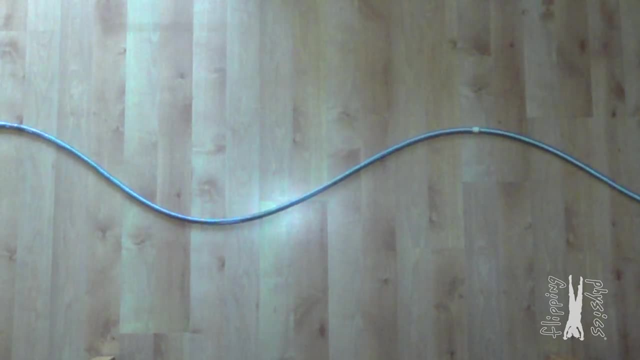 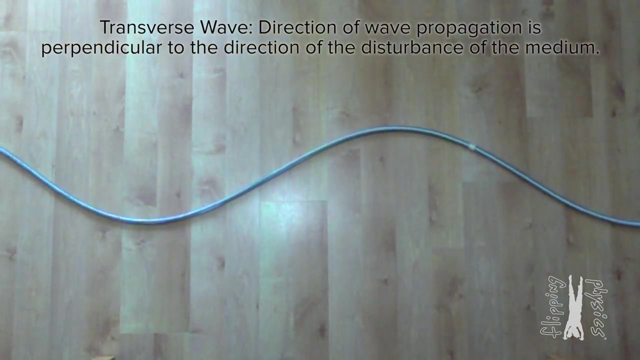 The wave we have been looking at this whole time is called a transverse wave. A transverse wave is where the direction of wave propagation is perpendicular to the direction of the disturbance of the medium. As you can see, the direction of wave propagation in this example is horizontal. 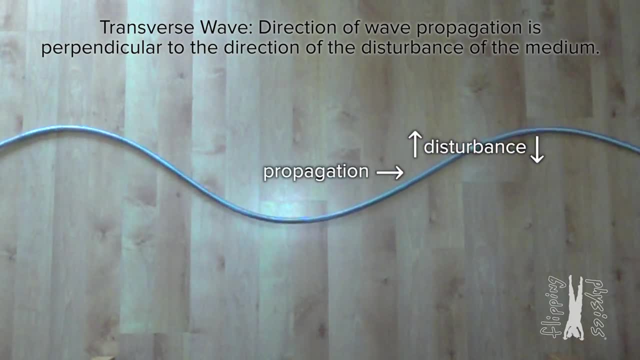 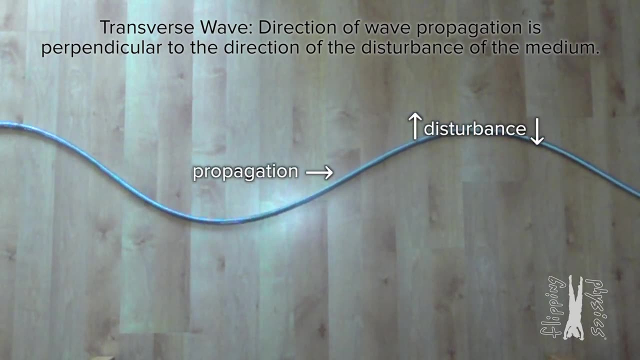 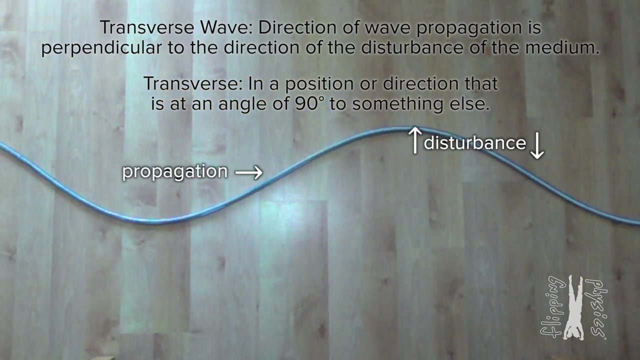 and the direction of the disturbance of the medium is vertical. Therefore, the direction of wave propagation is perpendicular to the direction of the disturbance of the medium. hence transverse wave, Mrp, And according to the Cambridge Dictionary, transverse means in a position or direction. 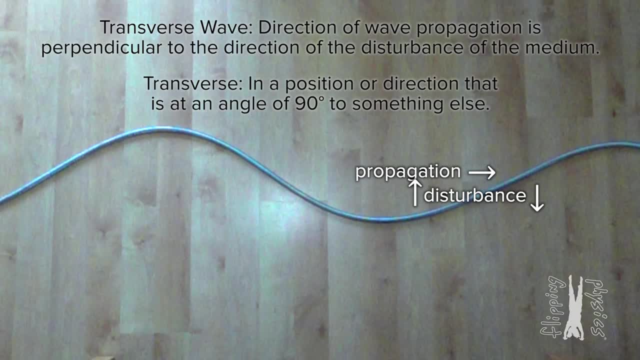 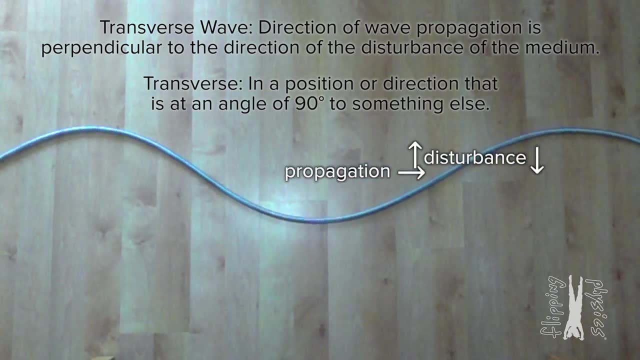 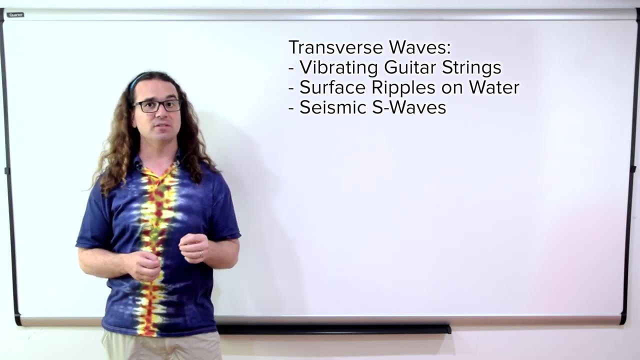 that is, at an angle of 90 degrees to something else. That must be why it is called a transverse wave. Billy, that is correct. Examples of transverse waves are waves on the strings of a guitar, ripples on the surface of a pond, seismic S-waves, which are waves in the earth. 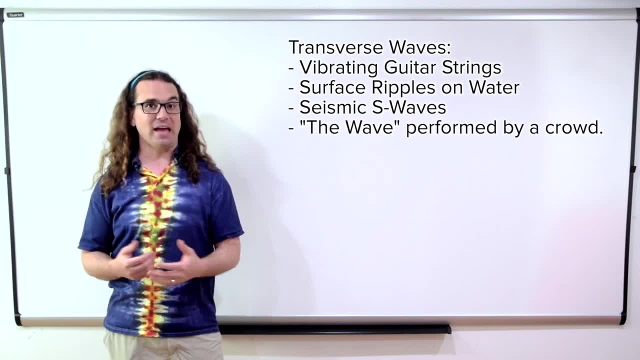 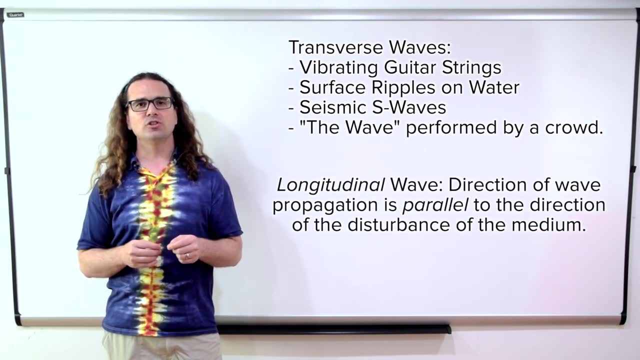 much like water waves and even the wave as performed by a crowd at a sports event. Now, the other type of wave is a longitudinal wave. A longitudinal wave is where the direction of wave propagation is parallel to the direction of the disturbance of the medium. 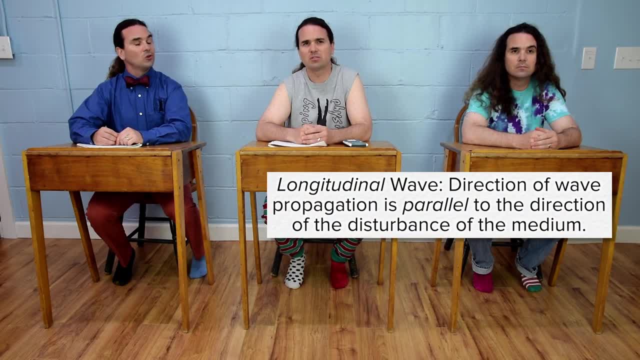 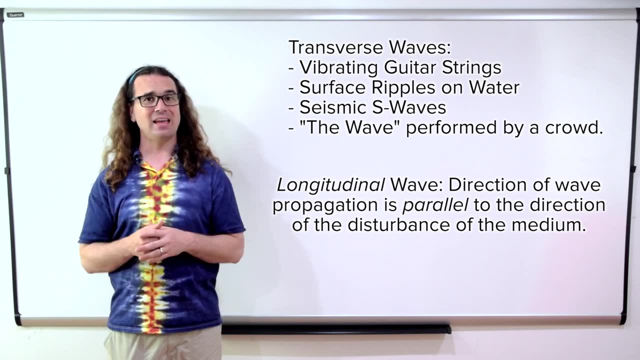 You just said the same thing as for a transverse wave, only you replaced perpendicular with parallel right. Bobby, that is correct. And in order to create a longitudinal wave on this spring, I grab the spring, compress it a bit and let go. 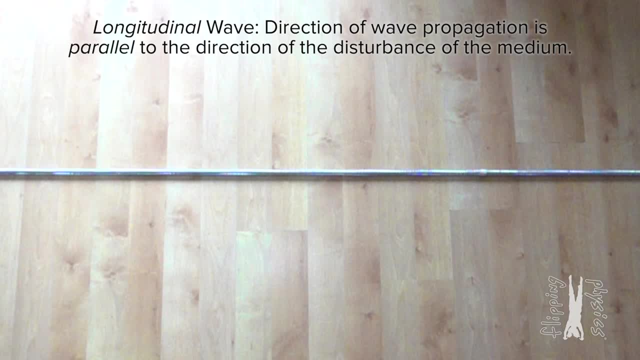 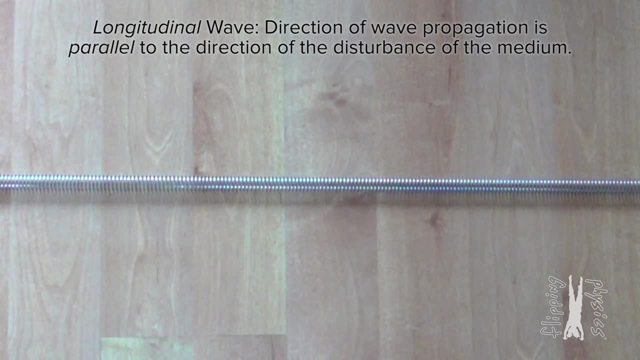 Uh… I don't see the longitudinal wave. Where is it, Mrp? Right, It is difficult to see, so let's zoom in a little bit. I still don't see it, Mrp, So it is difficult to see longitudinal waves on this spring. so I'm going to change. 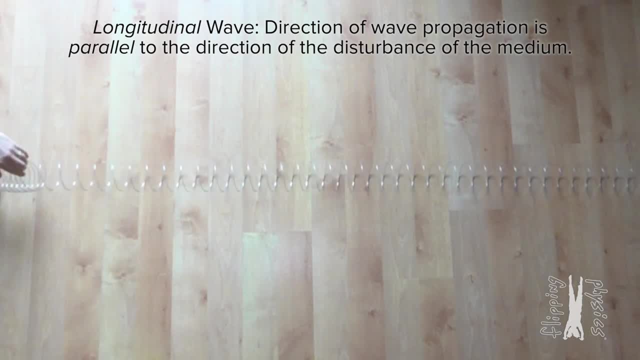 to demonstrating longitudinal waves on a slinky. I reach down again and compress a portion of the slinky and let go And you can see a wave pulse of compressed slinky travels horizontally and the direction of wave propagation is also horizontal. In other words, this is 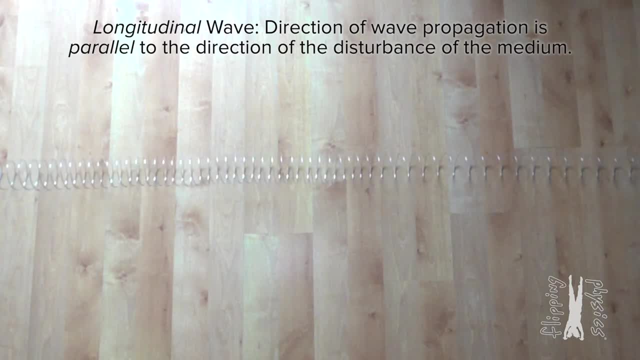 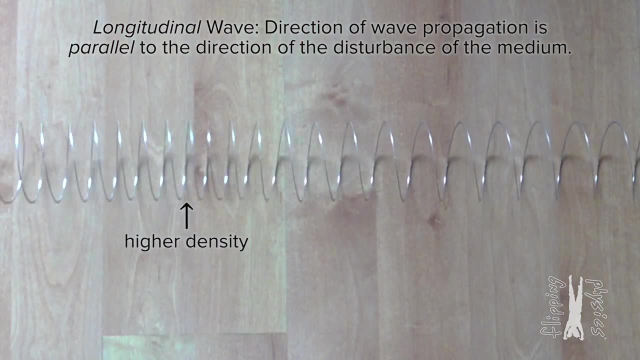 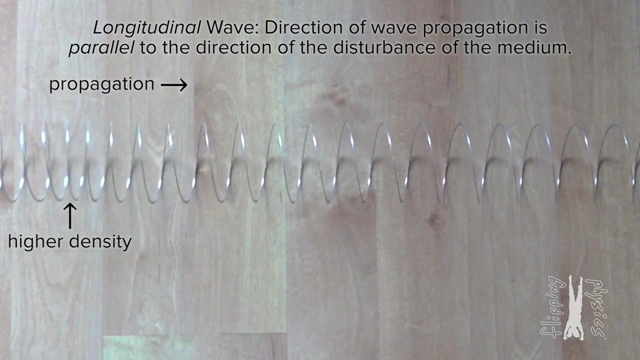 a longitudinal wave because the direction of wave propagation is parallel to the direction of the disturbance of the medium. And when we zoom in a bit you can see that compression or high density section of the spring move from left to right in the spring. Uh, rather than compressing the spring and then releasing it, could you push it in? 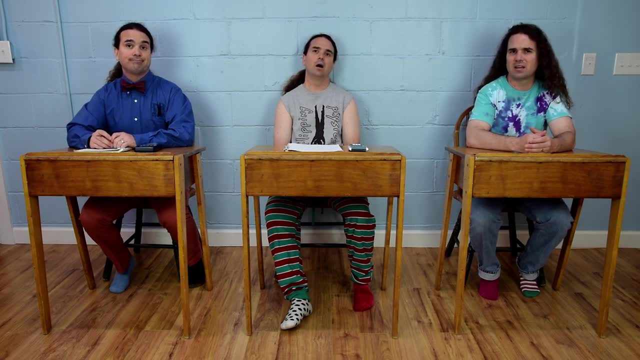 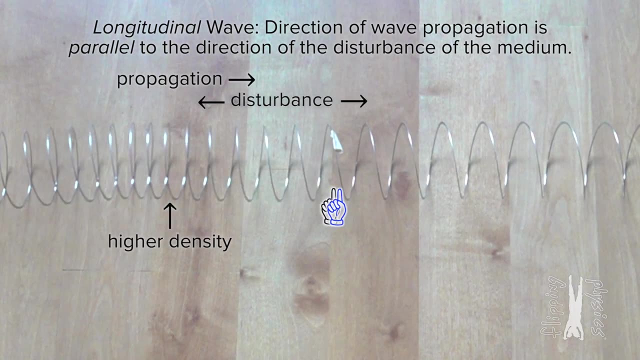 and then pull it back to create a full wave pulse instead of just a half wave pulse, Mrp. Good point, Bo. I can do that. Mrp, This is what a full longitudinal wave pulse looks like. I have added a piece. 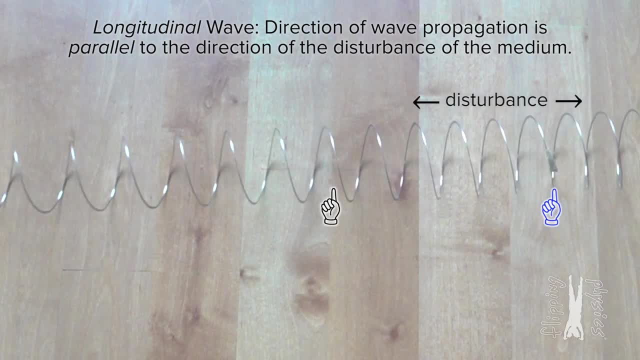 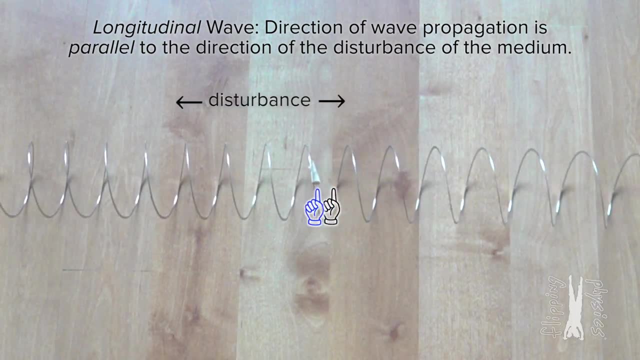 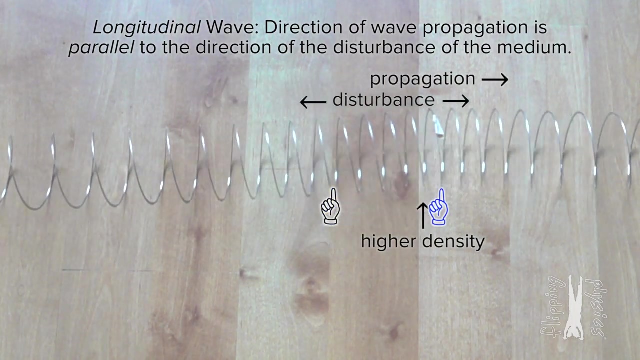 of tape so you can see the spring does come back to its original position, making the overall displacement of this wave equal to zero, or at least pretty close to zero. Again, this is called a longitudinal wave Right, because according to the Cambridge dictionary, longitudinal means lengthwise. 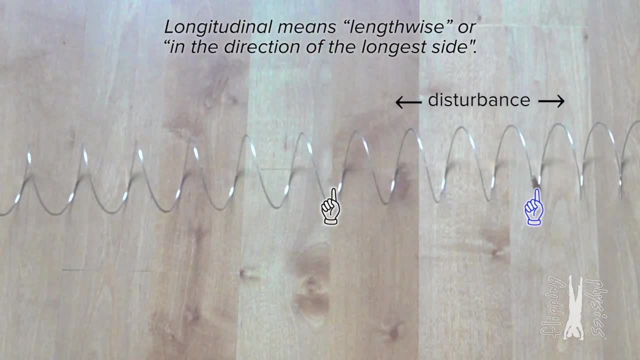 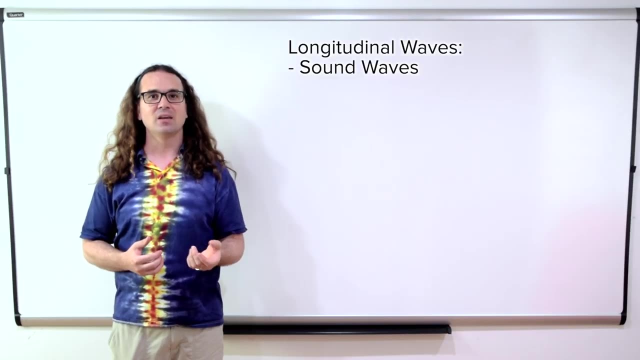 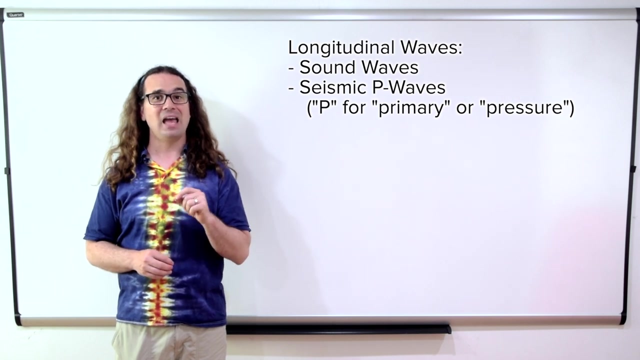 or in the direction of the longest side, which means parallel. Mrp. Yeah, close, Correct, Billy. Mrp, Exactly, Examples of longitudinal waves are the sound waves you use to hear me and seismic P waves. P is for primary or pressure wave. Seismic P waves are waves of high and low compression. 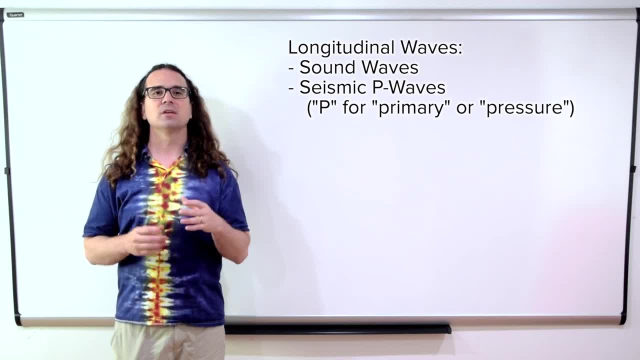 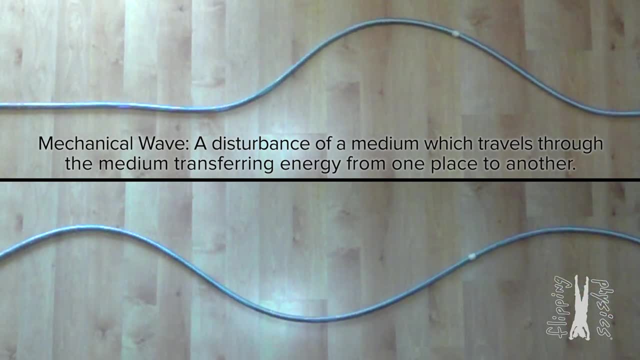 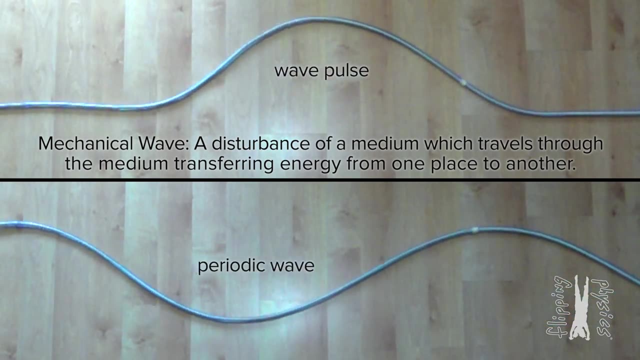 moving through the earth much like sound waves do. To review, we learned that mechanical waves are disturbances of a medium which travel through the medium, transferring energy from one place to another. We can have a single wave pulse or periodic waves, Which are continuous wave pulses. 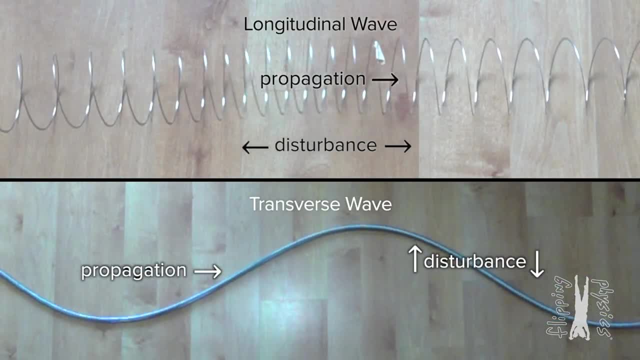 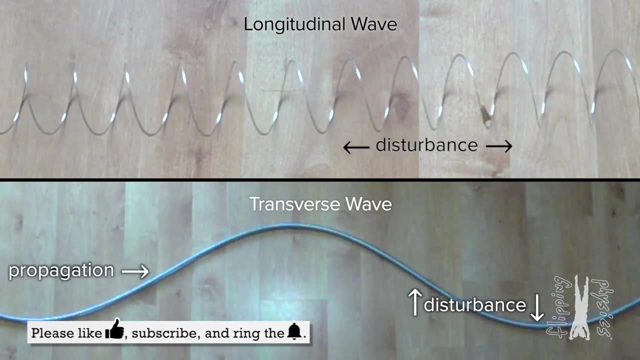 And there are two different types of mechanical waves: transverse and longitudinal. The difference has to do with how the disturbance of the medium moves relative to the direction of wave propagation. In a transverse wave, the two are perpendicular to one another. In a 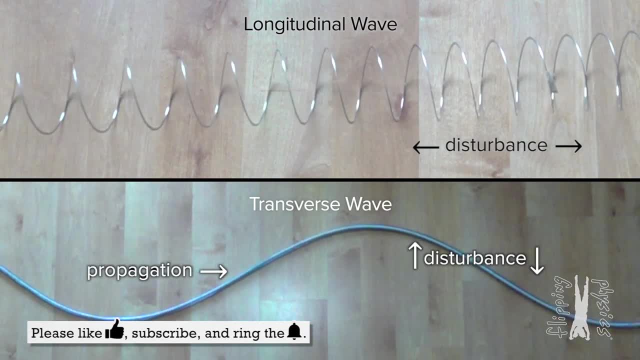 longitudinal wave. the two are parallel to one another. Thank you very much for learning with me today. I enjoyed learning with you.